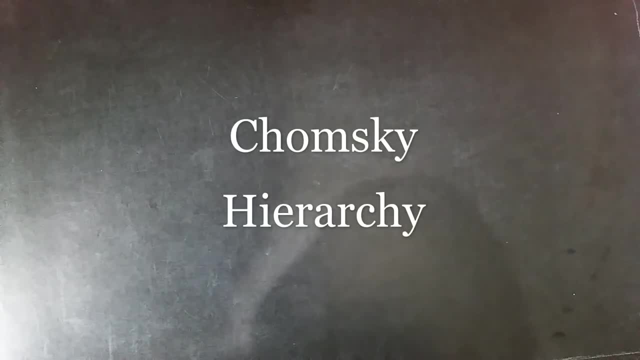 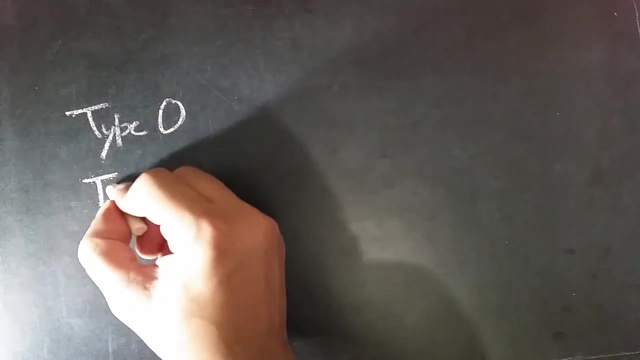 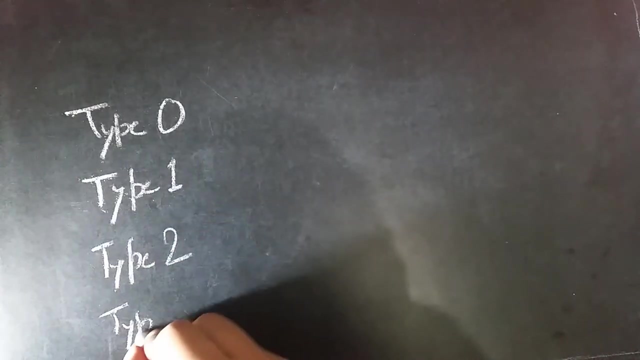 Hi everyone. today we are going to be talking about Noam Chomsky's classification of languages. Now, according to Noam Chomsky, there are four types of grammars. Those are type 0, type 1, type 2 and the last is type 3.. 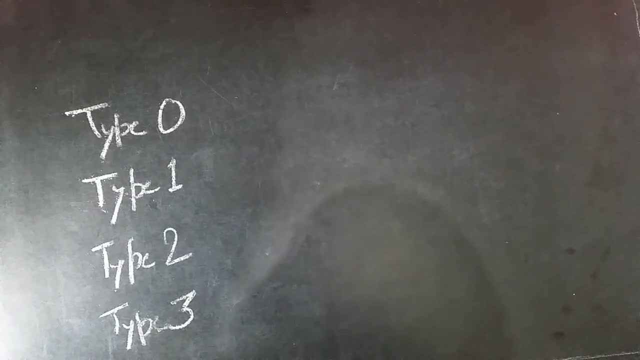 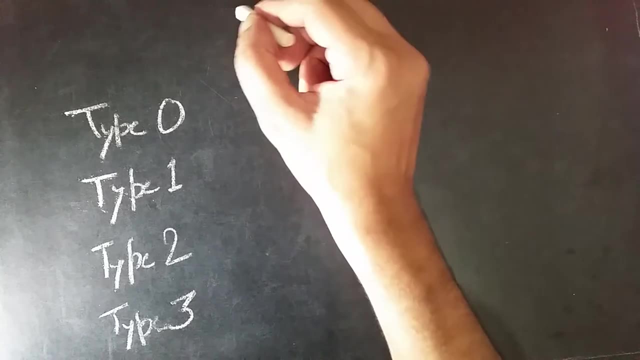 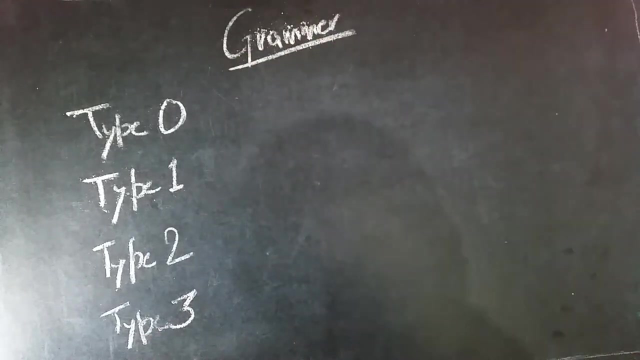 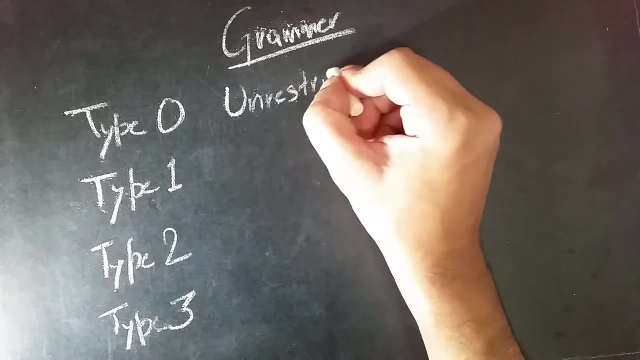 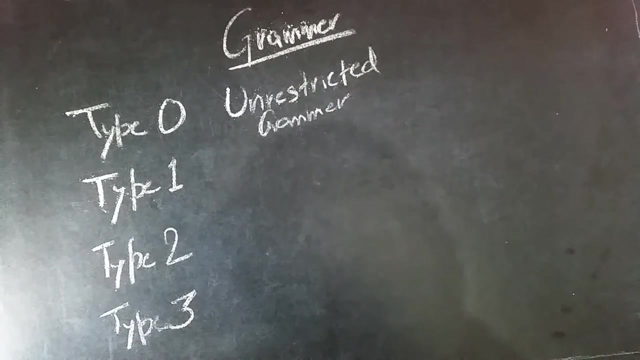 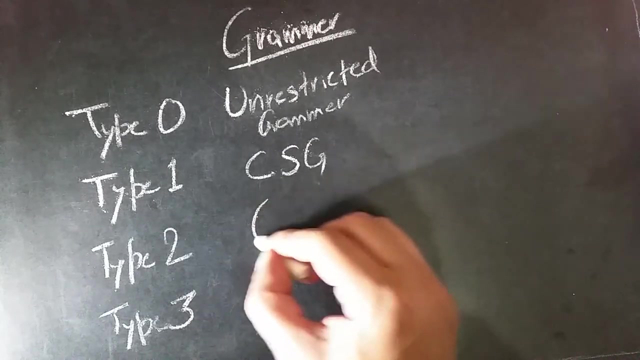 Now what's the difference between them is on the basis of grammar accepted, language accepted and the corresponding automata. So first let's see the grammar accepted. So grammar accepted by type 0 is unrestricted grammar. Grammar accepted by type 1 is context sensitive grammar. Grammar accepted by type 2 is context free grammar. 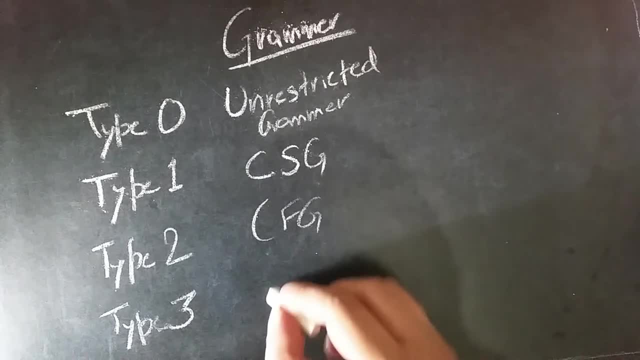 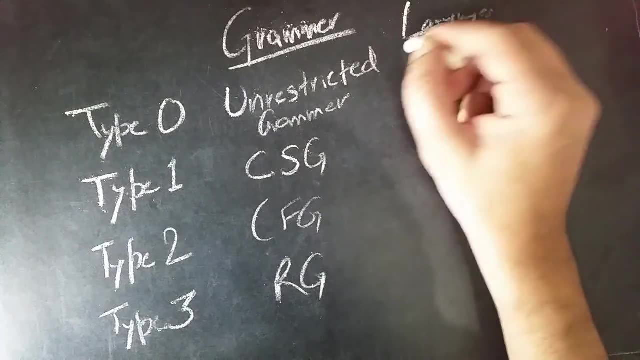 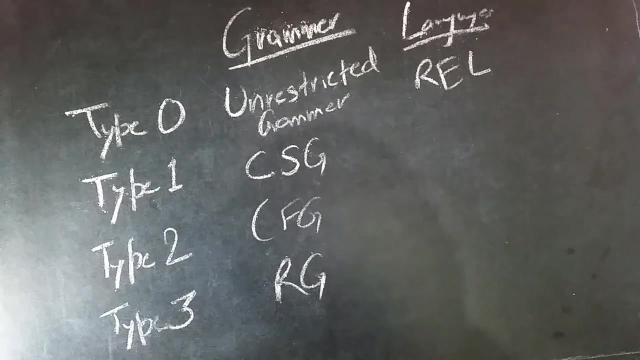 And the most restrictive of them all. the type 3 is regular grammar. Similarly, the languages accepted would be: by type 0, it's recursive enumerable language. By type 1, it's context sensitive grammar. By type 2, it's context free language. 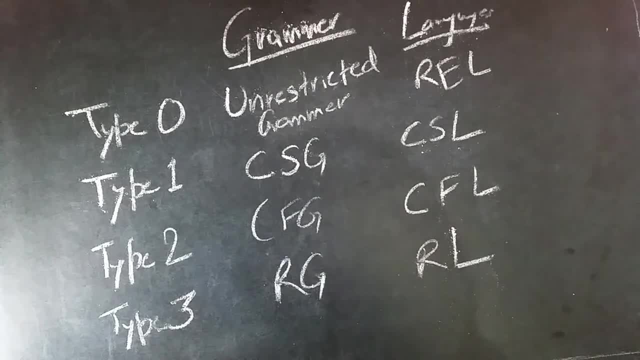 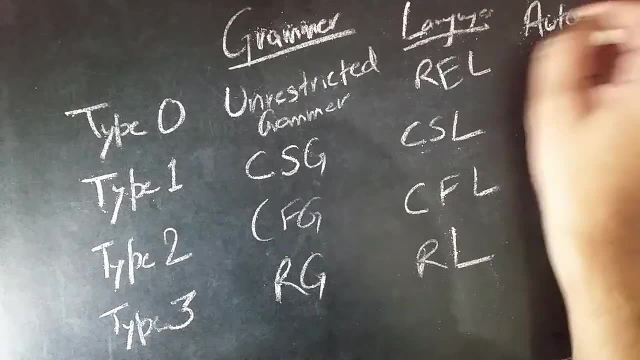 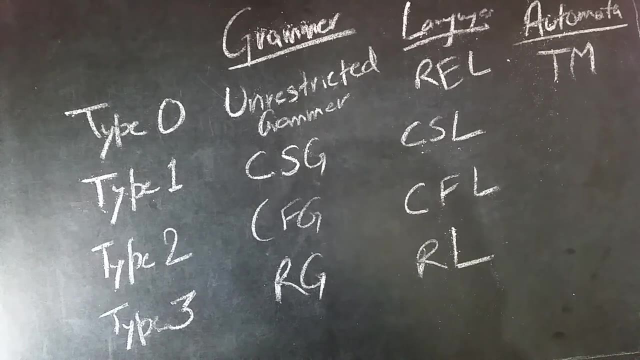 And by type 3, it's regular language, Same for corresponding automata. By type 0, the automata is Turing machine, the most powerful of them all. By type 1, it's linear bounded automata which, by the way, is not in gate syllabus. 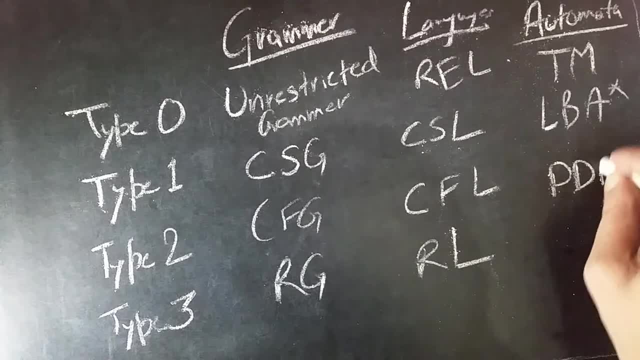 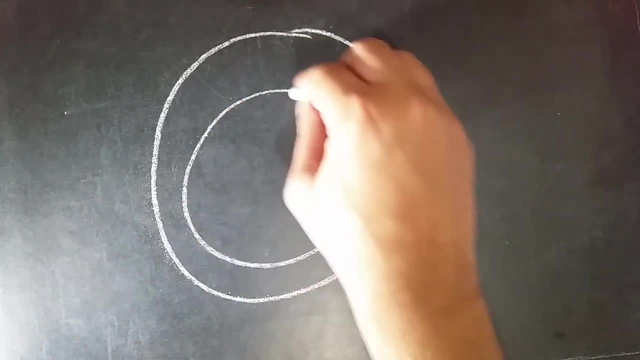 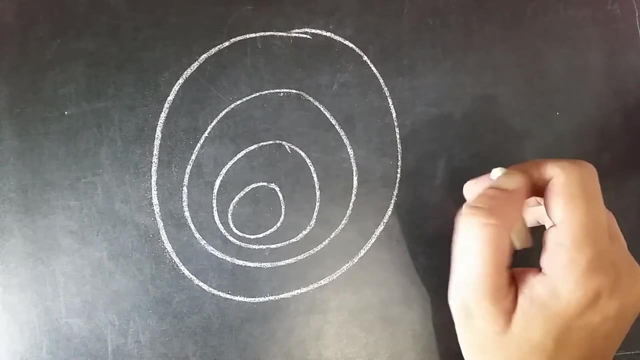 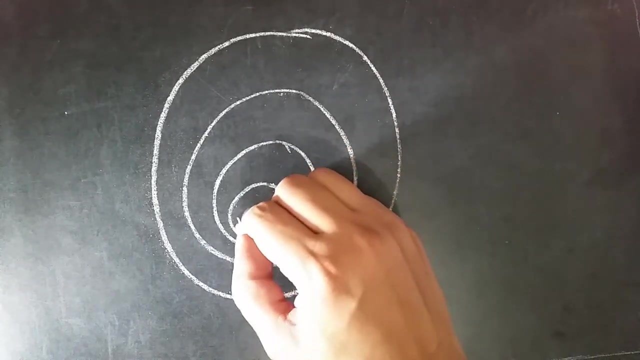 By type 2, it's pushing- It's pushed down automata. And by type 3, it's finite automata. It shows that out of all the four types of the grammars, each one is enclosed within the other. So the type 3, or regular, is the most restrictive of them all. 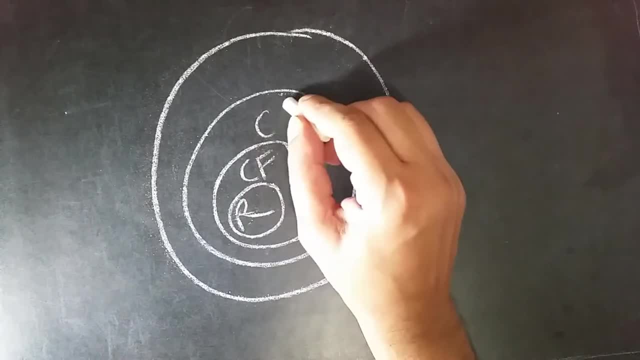 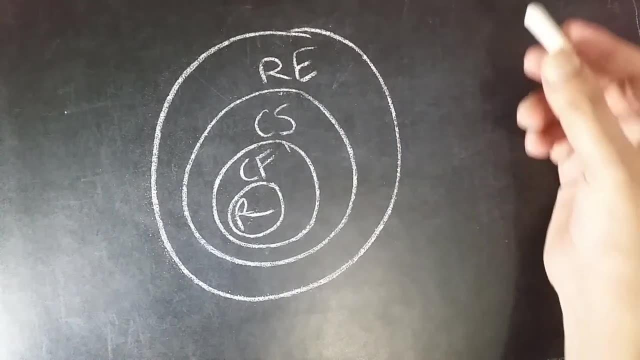 Its scope is least. Then come context free, Then context sensitive, And the recursive enumerable has the widest scope of them all. Or the powers, you could say where the type 0 has the highest power and type 3 has the least power of them all. 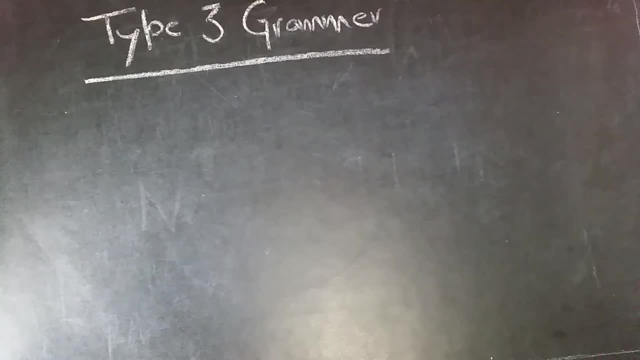 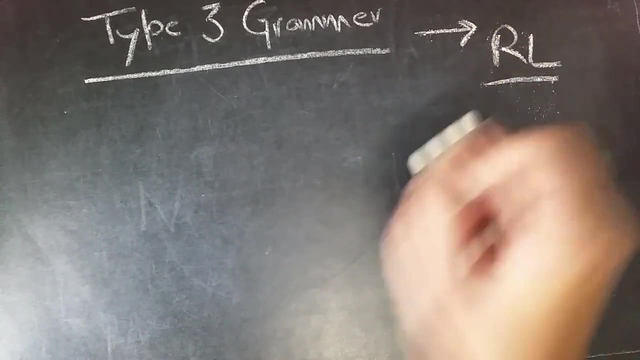 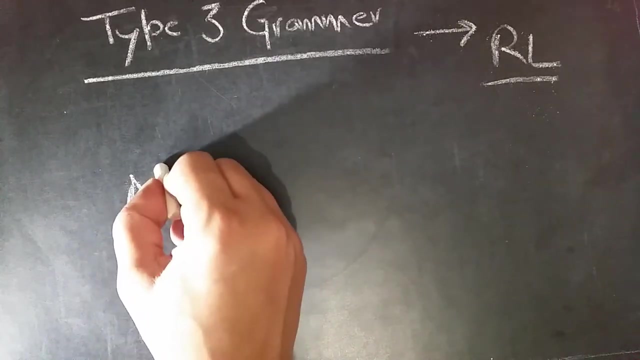 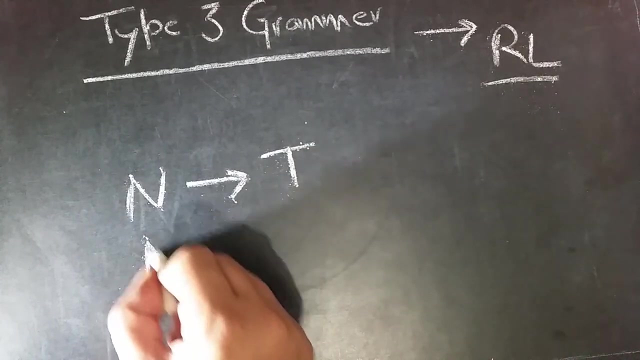 Now let's see each of them in detail. First let us see type 3 grammar. Now type 3 grammar. they generate regular language. Type 3 grammar must have a single non-terminal on left-hand side and right-hand side, consisting of a single terminal or a single terminal followed by a single non-terminal. 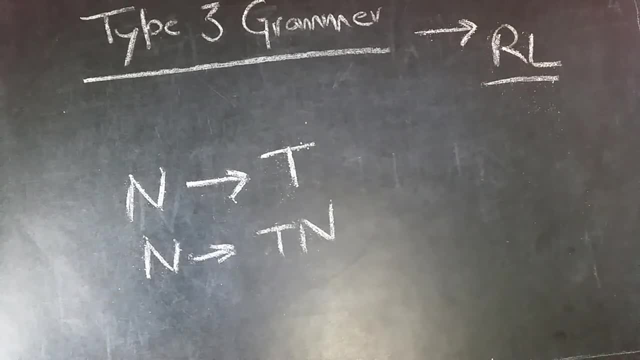 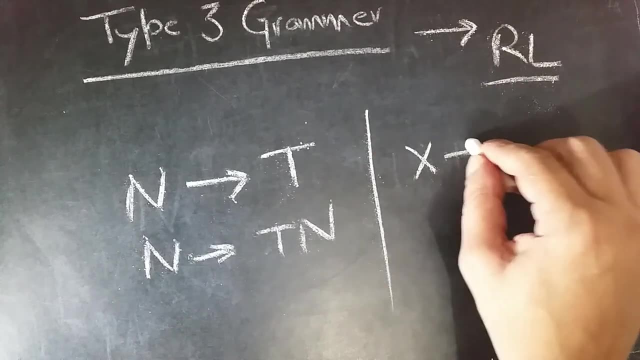 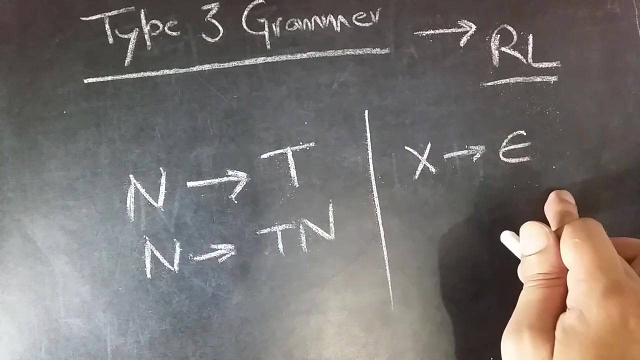 These are the only two productions that are allowed in type 3 grammar. It is most restrictive of them all. So you can give examples such as: x gives epsilon. This is allowed if x does not appear on right side of any rule. only in that case. 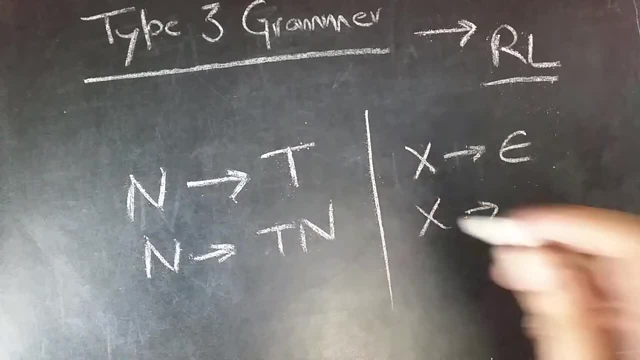 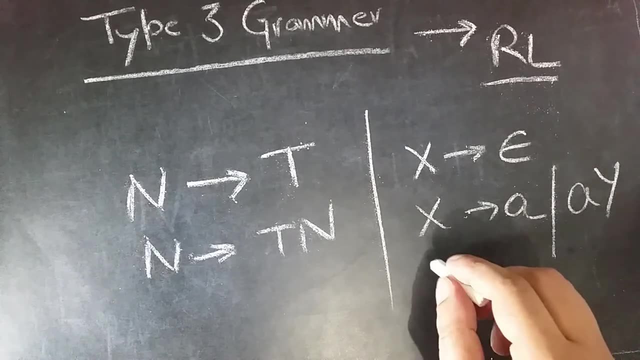 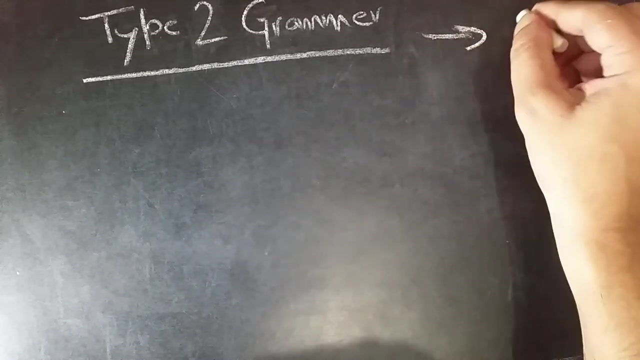 Or x can give a, so the first one would be a single terminal. This is allowed, Or a single terminal, followed by a non-terminal or just a single terminal. Now let us see type 2 grammar. As I said before, type 2 grammar: they generate context-free languages. 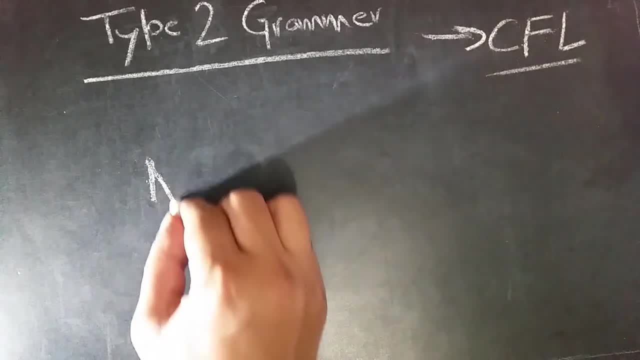 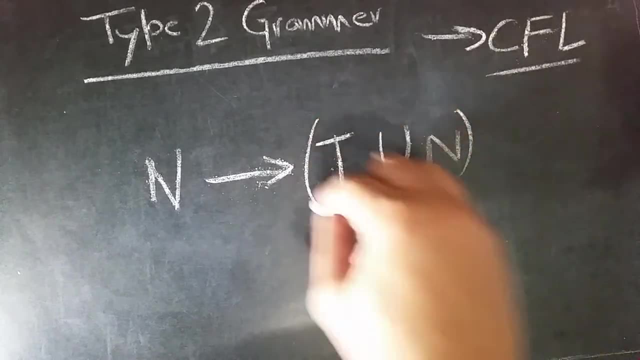 The production is of the form: a non-terminal produces a string of terminals and non-terminals, The languages. these languages generated by these grammars are recognized by non-deterministic post-term automata, as I have shown in the table before. So examples could be. 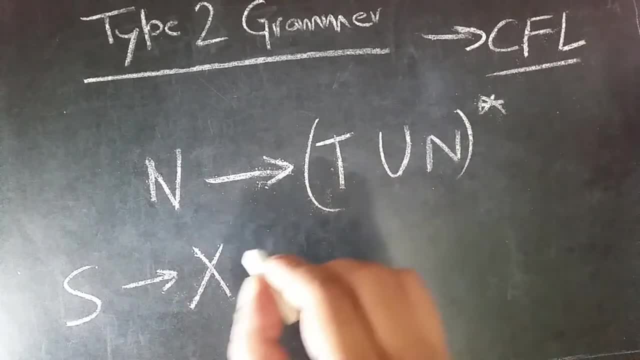 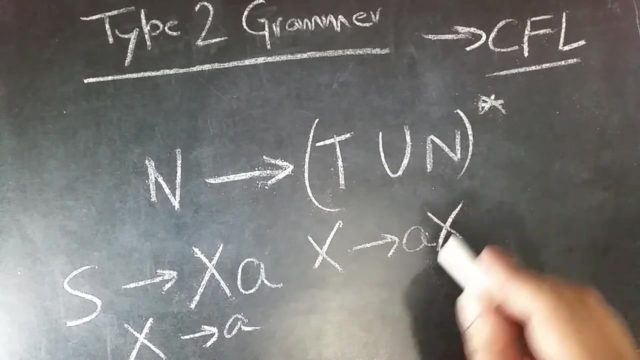 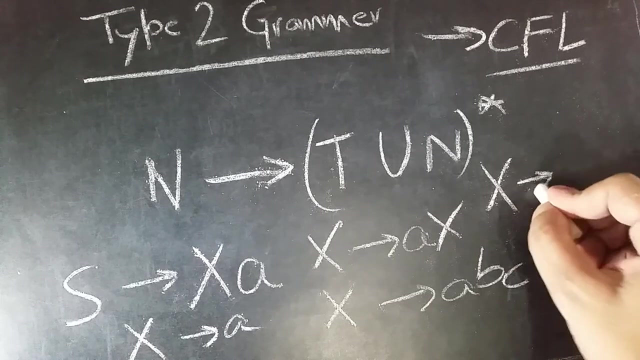 This is a non-terminal. It generates a non-terminal, followed by a terminal Or a non-terminal. it generates a terminal Or a non-terminal. it generates a terminal and non-terminal. A non-terminal generates a string of terminals Or a non-terminal. it generates epsilon. 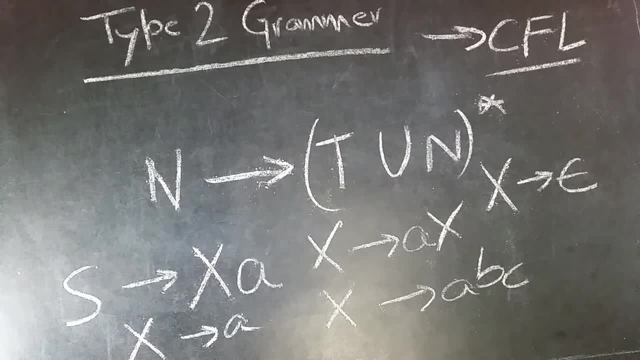 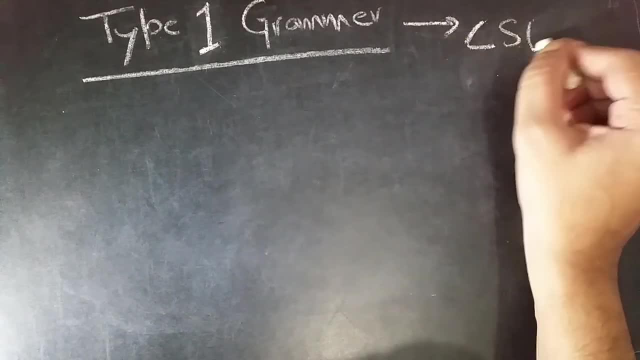 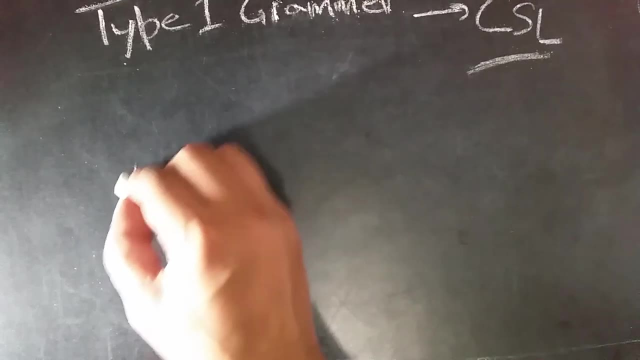 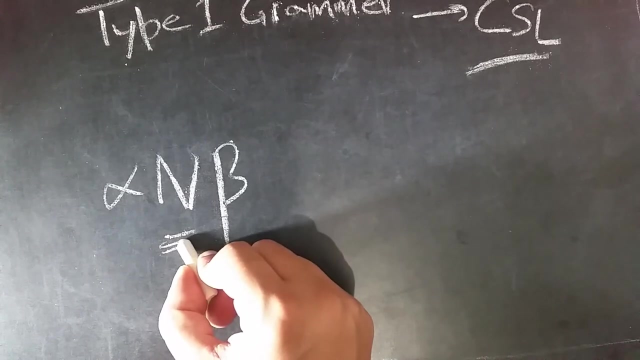 Now let us see type 1 grammars. Type 1 grammar, as I said before, generates context sensitive languages. Now the production must be of the form a string of terminals and non-terminals, but one non-terminal is a must, produces another string of non-terminals.